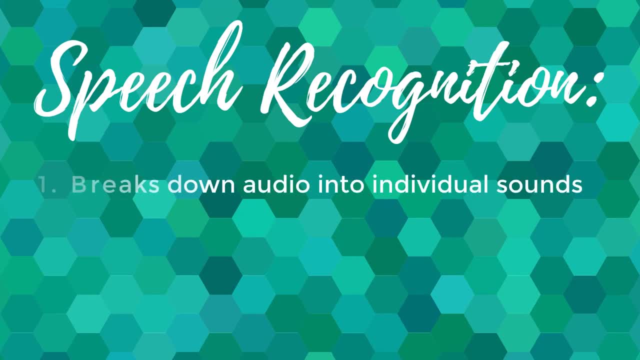 Well, speech recognition works by breaking down audio into individual sounds, converting these sounds into a digital format and using algorithms and models to find the most probable word fit in that language. To better understand this, let's dig deeper on each of these steps. 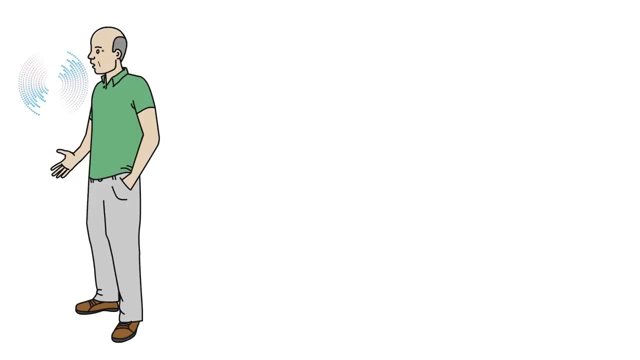 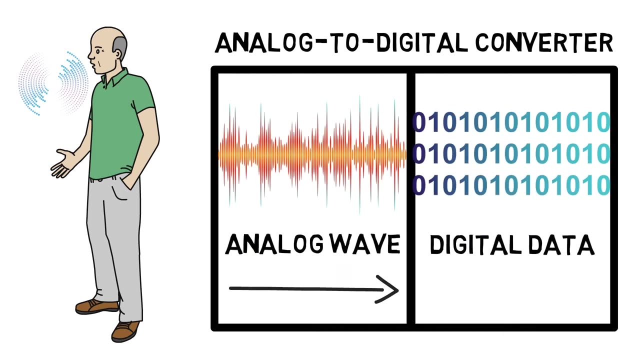 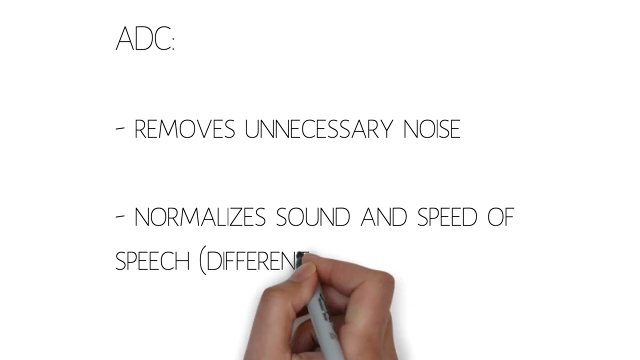 To better understand this, let's dig deeper on each of these steps. So when people speak, they create vibrations in the air. A device known as the analog-to-digital converter transforms the sound wave into binary data that the machine can understand. The ADC also filters the sound to remove unnecessary noise and normalizes the sound and speed of the speech to match the pre-recorded samples in the machine's device. 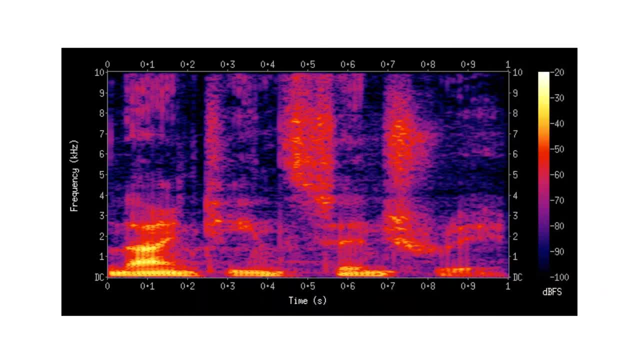 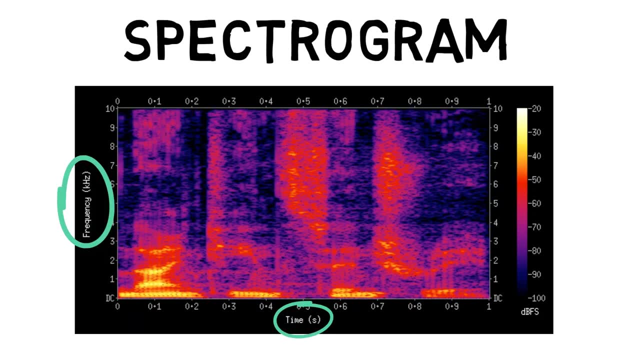 It then separates the data into different bands of frequency which the spectrogram then analyzes further. On the x-axis, there is time. On the y-axis, there is time. The y-axis plots the frequency of a sound, as in high pitches versus low pitches. 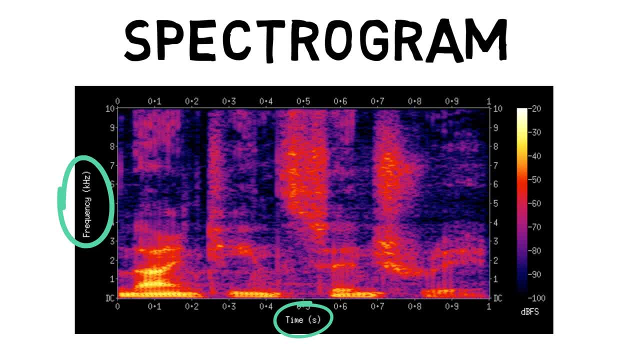 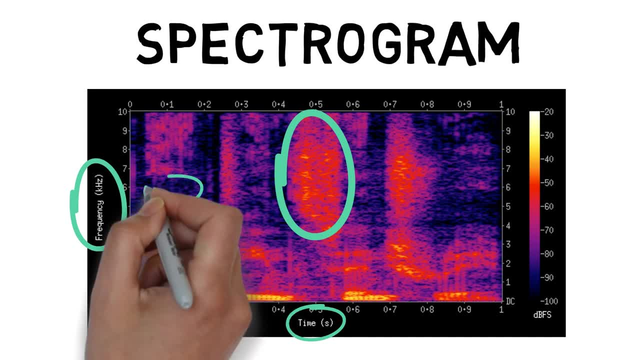 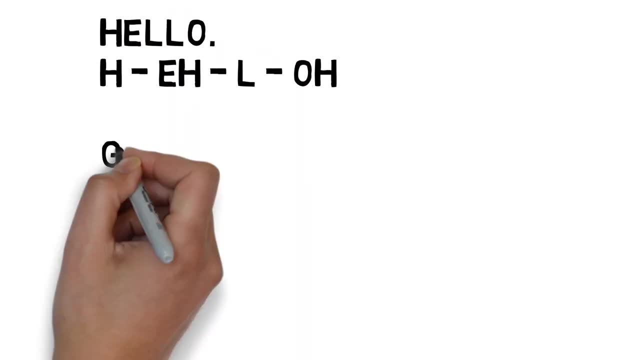 You see, all words are made up of distinct vowel sounds. They each have different frequencies which are recorded on this device. The areas that are brighter signify high frequencies and the areas that are darker signify low ones. All vowel sounds have different frequency patterns which can be pre-programmed into the computer, allowing it to recognize when a spoken sound matches a specific vowel sound. 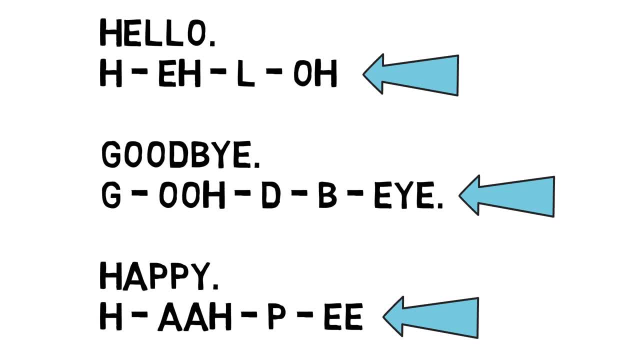 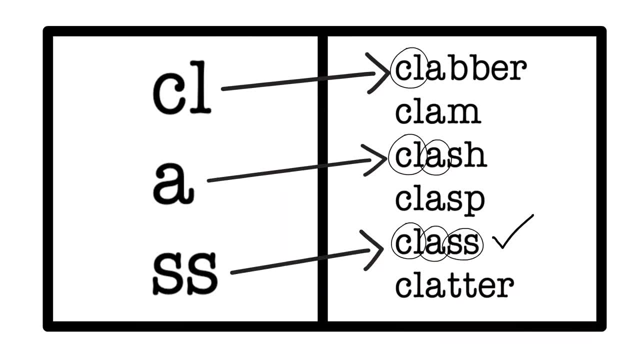 These here are known as phonemes, which are the smallest elements of a language that can be programmed into the computer. These here are known as phonemes, which are the smallest elements of a language that can be programmed into the computer. The computer then runs these phonemes through complex models that compare them to words in its pre-built dictionary. 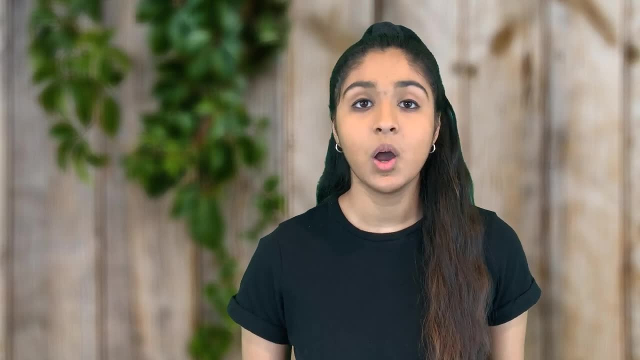 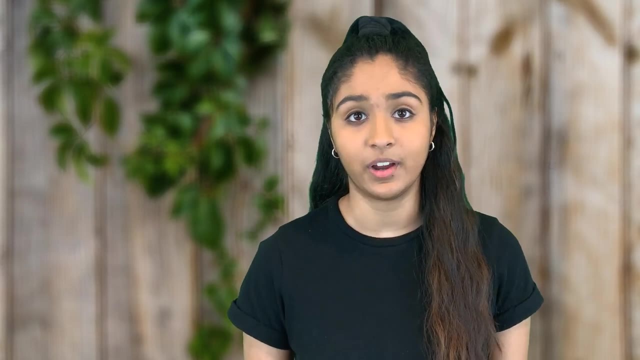 But there's a catch: Human language isn't so simple. We all know that humans speak with different accents, slangs, mispronunciations, and these variations aren't in a computer's dictionary. Well, this is where models such as the Hidden Markov Model come in. 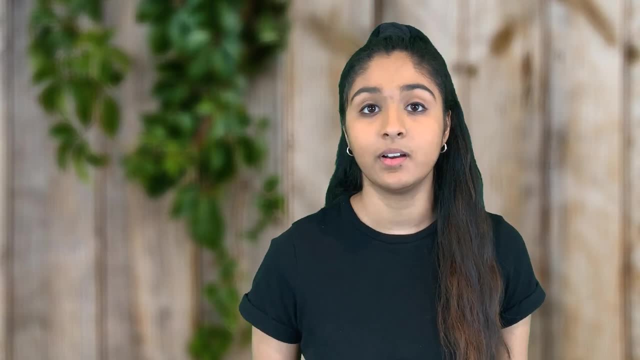 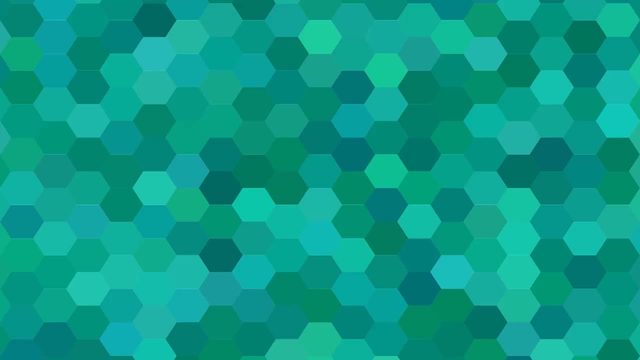 But for now, just know that speech recognition uses models such as the Hidden Markov Model to understand the intricacies of our human language. Now let's look at another example. I saw a case study on Coursera on how a smart speaker works, and I 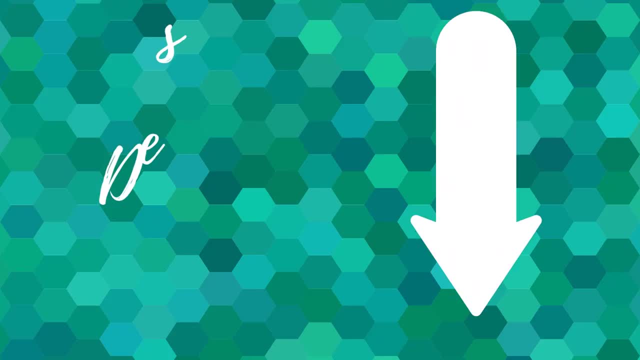 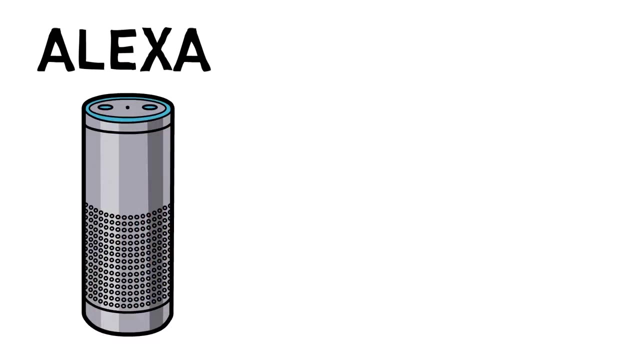 want to walk you guys through this. if you'd like to check out this course, I've included a link to it in the description. Let's walk through exactly how Alexa works, which can be broken down into four steps. So let's say that you want Alexa to tell you a joke. 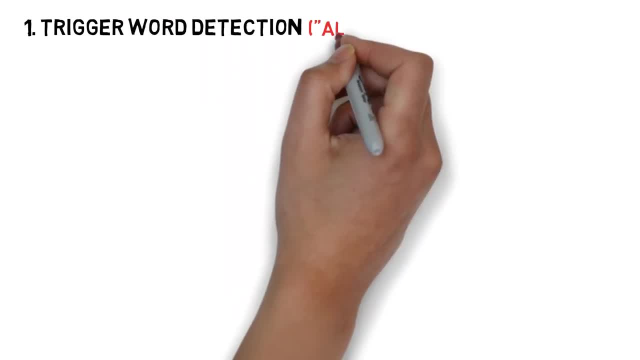 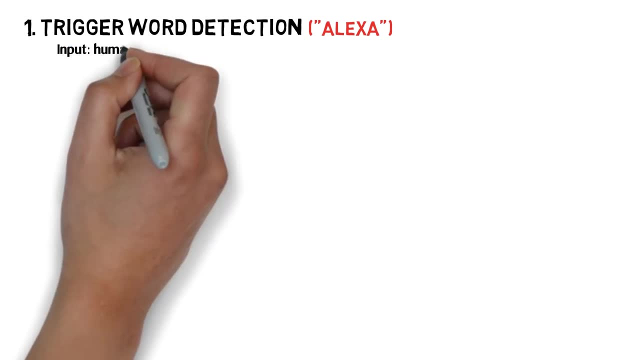 The first step is trigger word detection, and in this case, that'd be Alexa. This means that whenever Alexa hears this phrase, it knows that a command is coming. next, Alexa is programmed with an algorithm that will take in a phrase said by the human as input and output, either a zero or one. 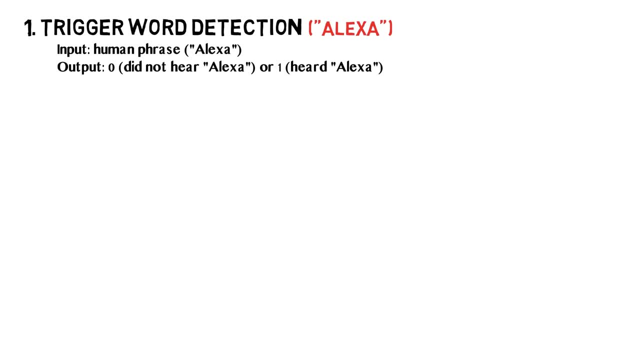 depending on whether or not the phrase matches alexa. next, alexa will use speech recognition to detect the next words after alexa. it will then translate this audio into a text transcript. intent recognition is the next step, which is where alexa will use nlp to figure out exactly what you. 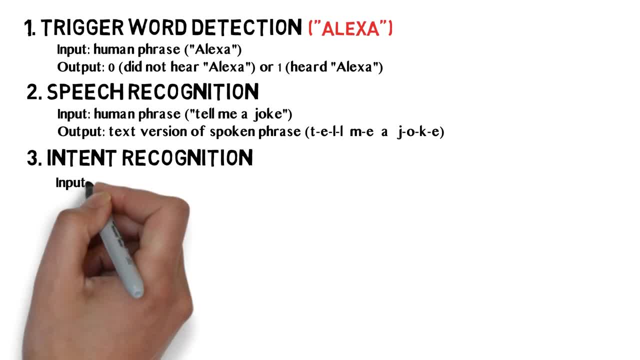 are telling it to do, or your intent. it will use another algorithm that takes in your words as input and matches it to one of the operations in a pre-programmed list. lastly, alexa will execute your command, in this case telling you a joke. to respond back with words, it would use speech. 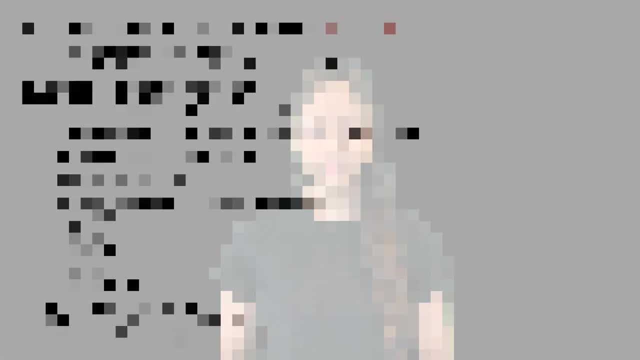 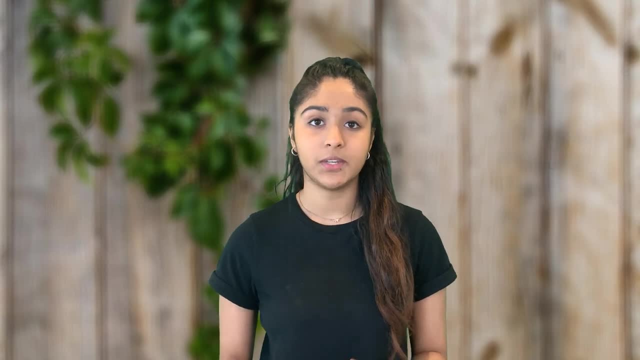 synthesis, which is essentially the opposite of speech recognition. so the next time you ask alexa to play some music or tell you a joke, you know exactly how she's doing it. now. alexa, as you know, is a bot that you can have voice conversations with, but there are also some virtual assistants. 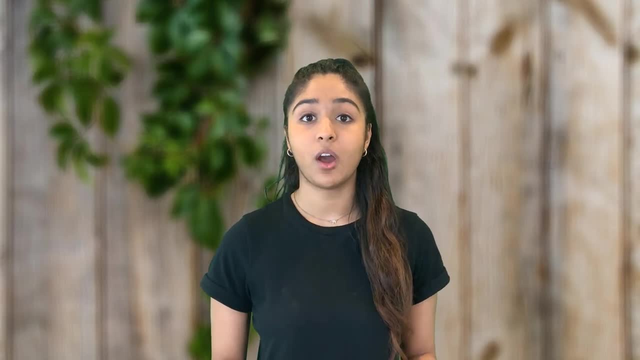 that you can chat with without any voice interaction, and these are the most important things that you need to know about alexa when you're trying to communicate with alexa, these are most commonly known as messenger chat bots. messenger chat bots are often easier and more effective to build as they don't require pre-recorded speech responses. 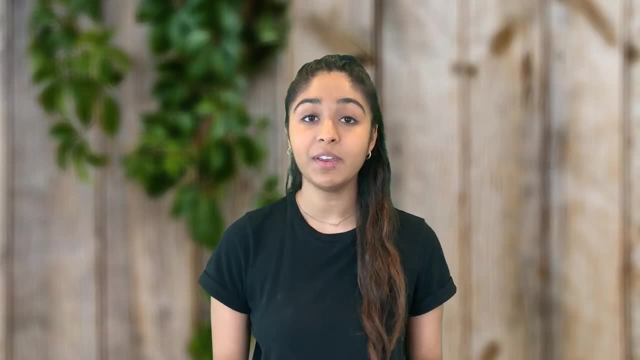 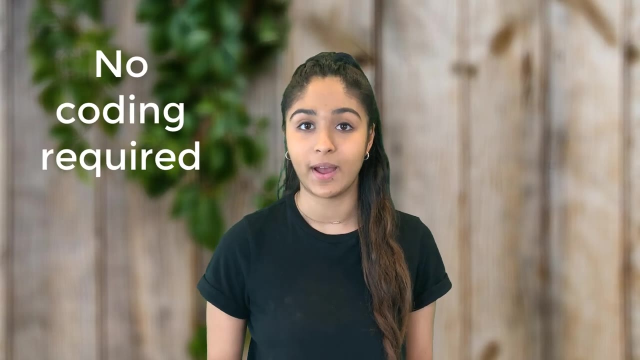 to user queries. so in the next few videos, i'm going to be introducing you to the world of chat bots as well as a free platform on which you can actually build one yourself, no coding required, and if you've enjoyed learning about speech recognition in this video, make sure to give it a thumbs up and 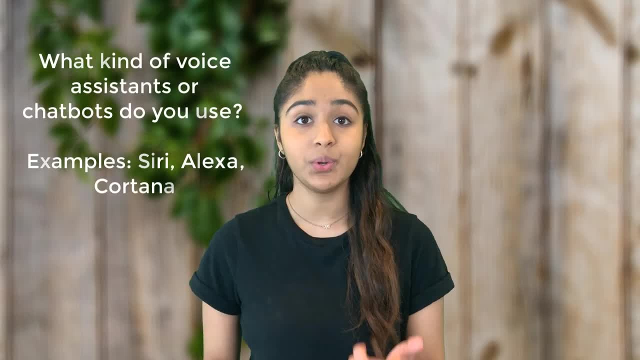 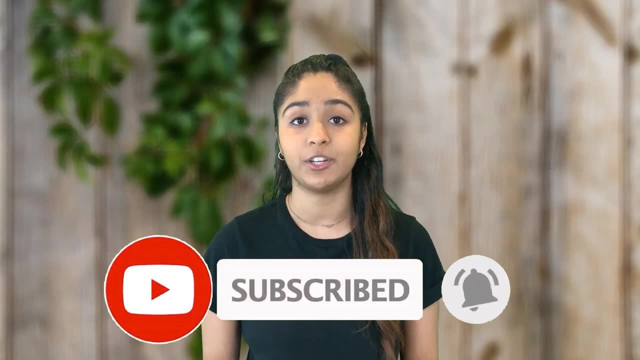 comment down below what kind of voice assistants or text chat bots you use in your daily life, and if you're new here, then make sure to subscribe and turn on notifications so that you don't miss any videos that will help you on your journey towards mastering artificial intelligence. thanks for watching and i'll see you in the next one.